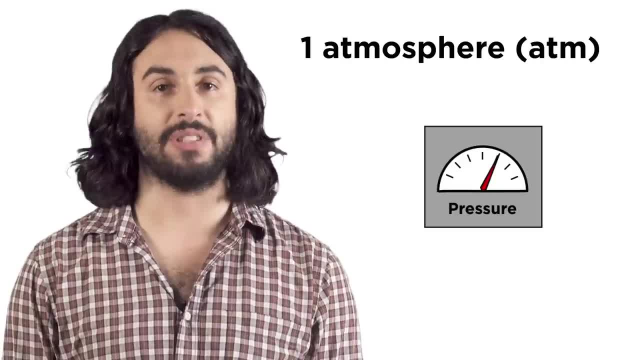 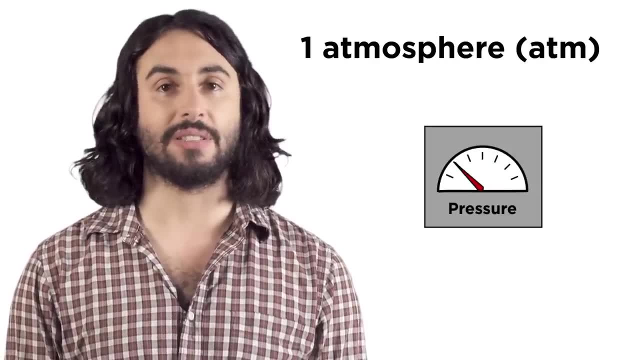 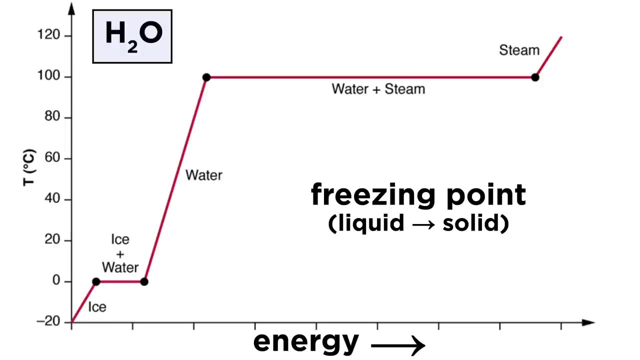 The normal boiling point of a liquid is measured at 1 atmosphere or the pressure at sea level. When atmospheric pressure decreases, the boiling point decreases, which is why water boils at a lower temperature. at higher altitudes, The freezing point of a substance is the temperature at which a liquid turns to crystalline. 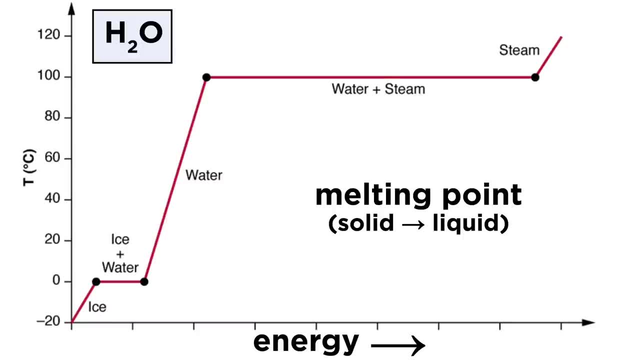 solid. The melting point is the temperature at which a crystalline solid melts. These are the same temperature. they just represent processes in opposite directions. As we heat a sample of ice, it will melt and then boil. On this diagram, the flat sections represent the phase changes themselves. 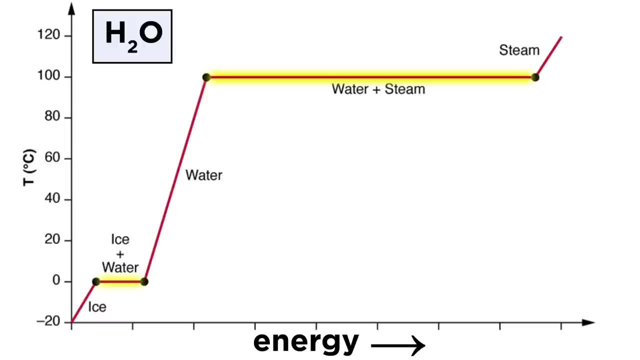 In these sections the temperature doesn't rise because the temperature is higher than the melting point, but because the heat energy being added is going towards disrupting the lattice energy of ice or overwhelming the hydrogen bonds occurring in liquid water. So during these periods the heat energy does not go towards heating the sample. 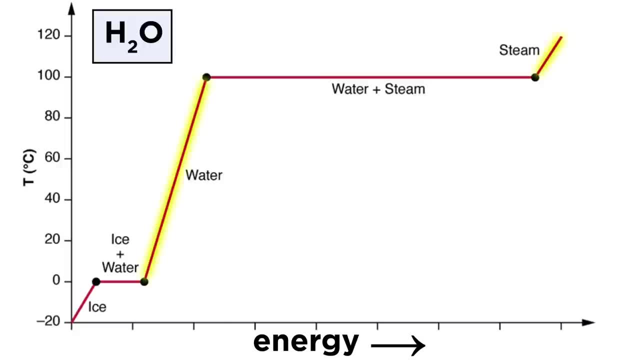 Once a phase change is complete, the heat energy returns to heating the sample. The energy exchanged during melting and boiling is called the heat of fusion and the heat of vaporization returns. The phase change is denoted by these subscripts telling us when water is considered solid. 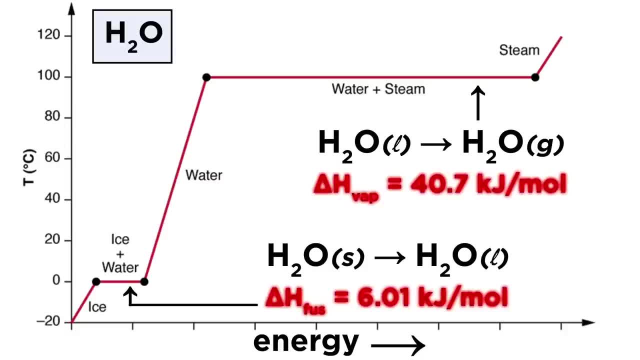 liquid or gas, and this is the energy needed per mole of water to cause the phase change. This is specific to water because every compound has a different lattice energy in the solid phase and makes intermolecular contacts of differing strength in the liquid phase. 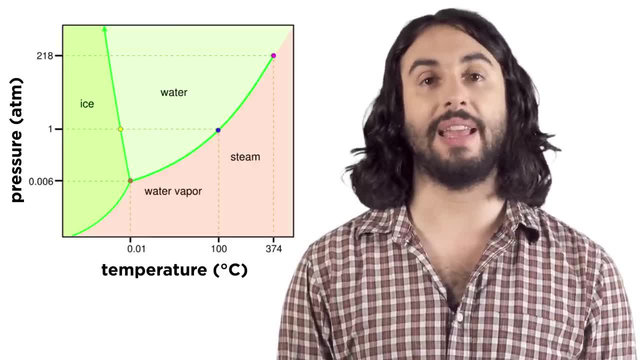 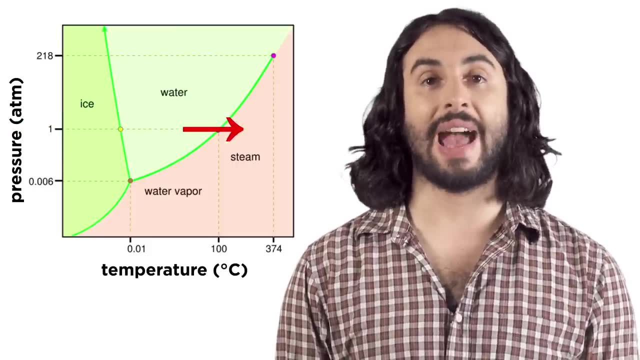 Phase diagrams show what phase a sample is. The phase diagram shows what phase a sample is. The phase diagram shows what phase a substance will be in at a particular temperature and pressure. For water, we can see the phases we would expect at atmospheric pressure. 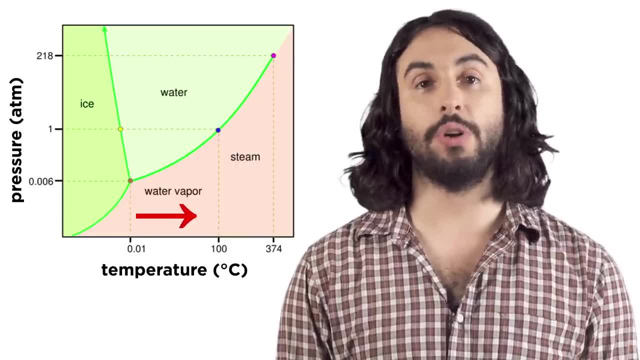 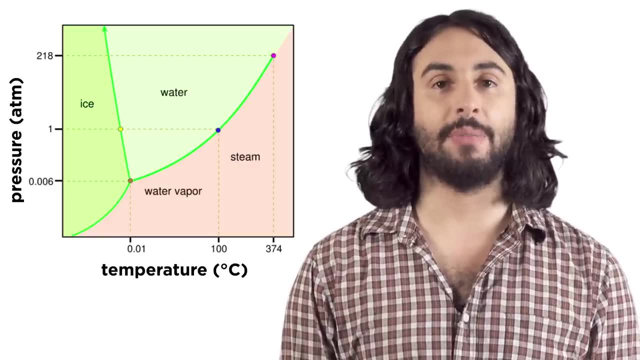 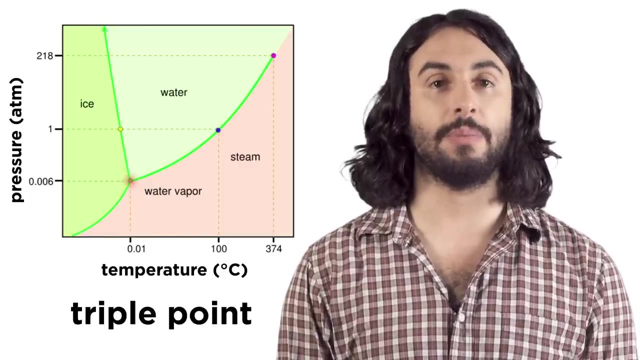 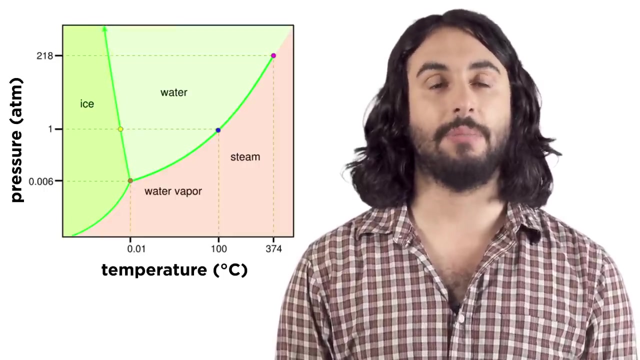 If the pressure is dramatically lowered, we can see how water would sublimate as the temperature increases, instead of melting first. On a phase diagram, lines represent equilibria between two phases and the triple point represents an equilibrium between all three. For water, the line between solid and liquid slants up and left because the solid form